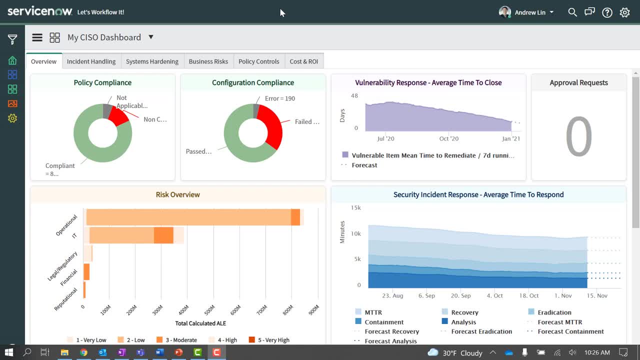 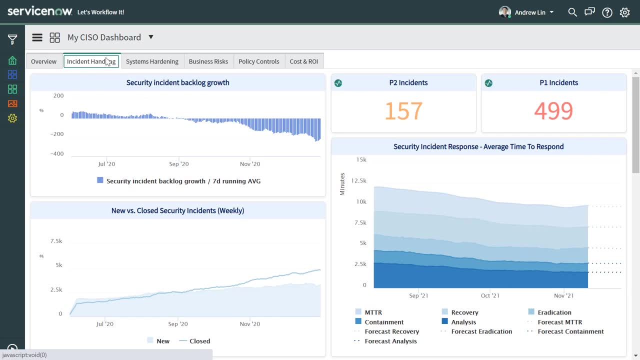 management, vulnerability response and security incident response. Dashboard tabs can be created to organize the data. In this example, the incident handling tab provides extra detail for different groups, but they can be arranged and styled however any individual user prefers. the now platform is now fully integrated with the MITRE. 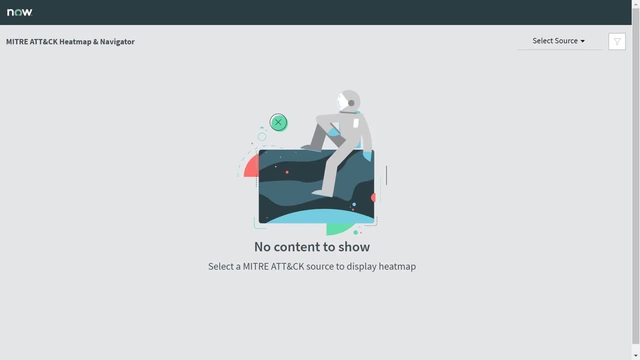 ATT&CK framework for threat intelligence, which can provide valuable insights that security professionals need to get work done better every day. MITRE ATT&CK can assist security leaders in managing security programs by helping them understand how the various defensive systems are performing and to identify where there might be any gaps. the MITRE ATT&CK heat map and navigator can provide. 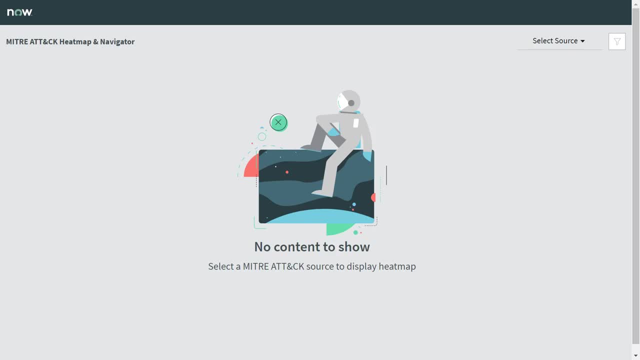 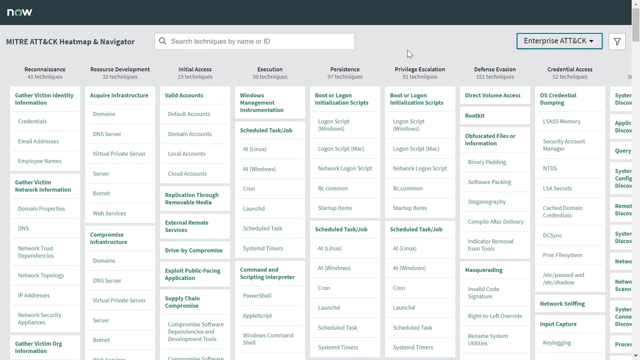 immediate visibility into patterns where the department is seeing any concentration of incidents or is dealing with any role relevant vulnerabilities. it also provides a quick visual of the current security posture for detecting and defending against each of these attack technique techniques. all of this helps the CISO understand where investments of time and resources are. 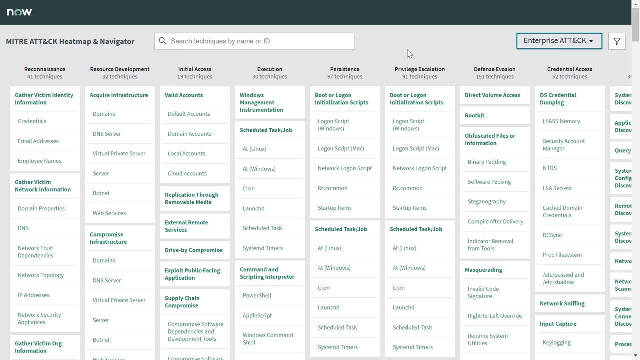 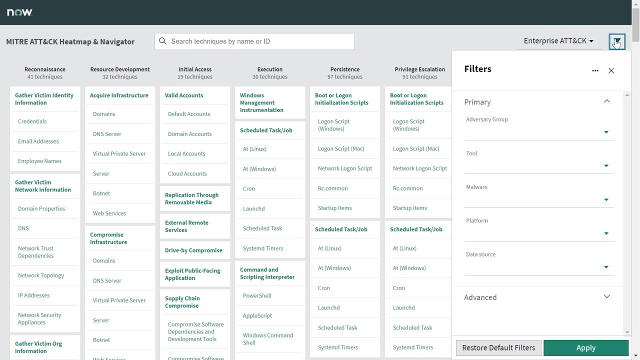 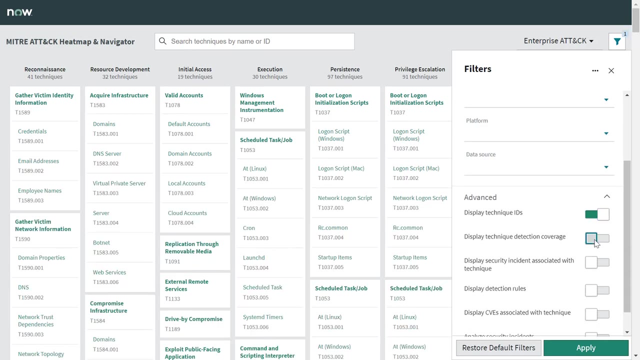 most needed here. we'll set some filters to show how the heat map and navigator functions watch as the changes occur. as we set those filters, the heat map will change as we do. so in this case I'm going to set the display technique IDs. display technique detection: coverage: display detection. 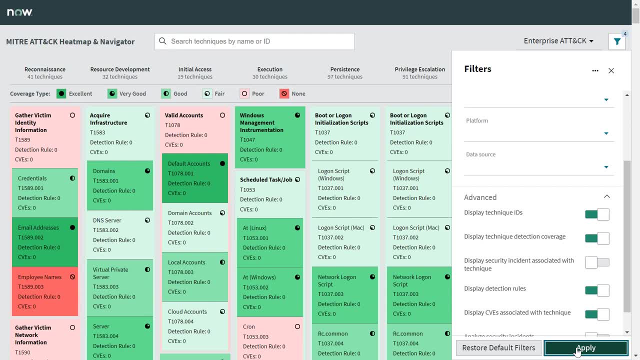 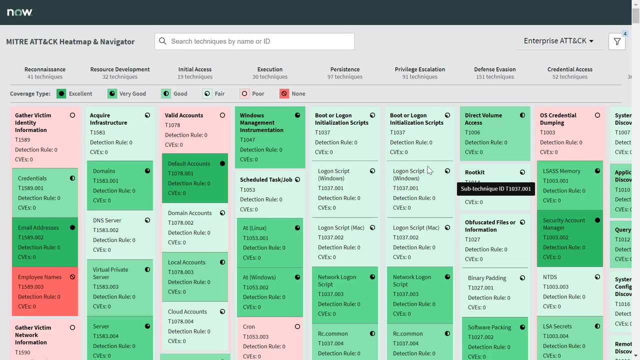 rules and display CBEs associated with technique. this is an extremely valuable resource when it comes to thwarting the attack patterns that impact and threaten the organization the most, such as those from advanced persistent threat groups like UNC 2452 during the SolarWinds breach. we'll set a filter. 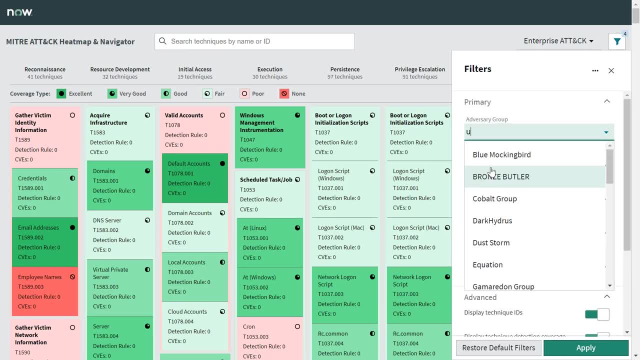 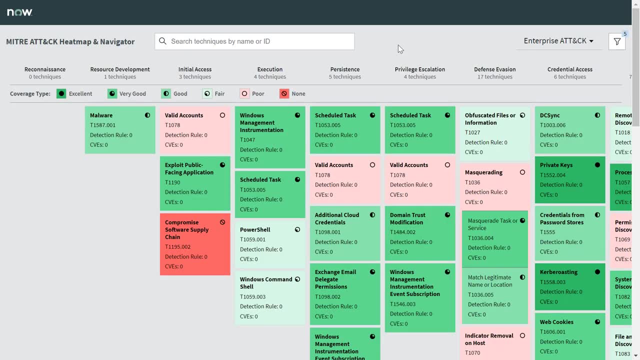 that is well at the very top. and the adversary group. we just start with UNC and then we go see the rest of the adversary group. we apply it and then you can see as we add in this final data point of the known adversary group. it draws in all the known techniques of this advanced, persistent threat, the CISO. 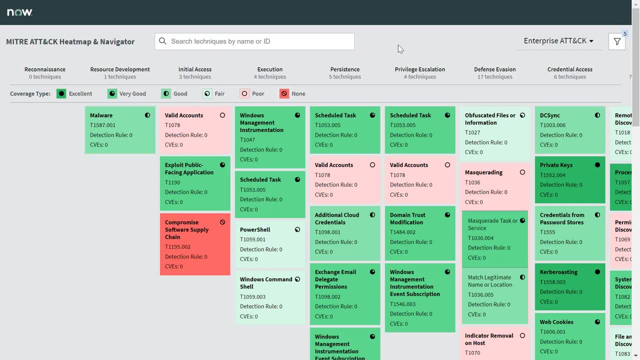 can then drill down to each of these, but, moreover, this shows the current organizational posture and defense against this known apt. so you can see that we're getting everything in one place. but you might be asking yourself: is there any value to all these other algorithms or things like that? 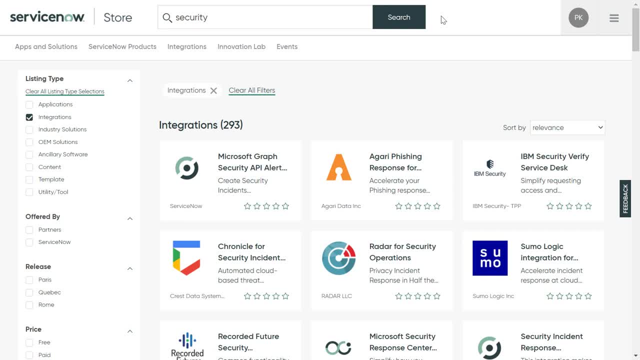 well, for one of the things we need to keep in mind is that there are some we might not want to figure out- all the things we need to figure out- but you might be asking yourself: how did we get here? It all starts with integrations. 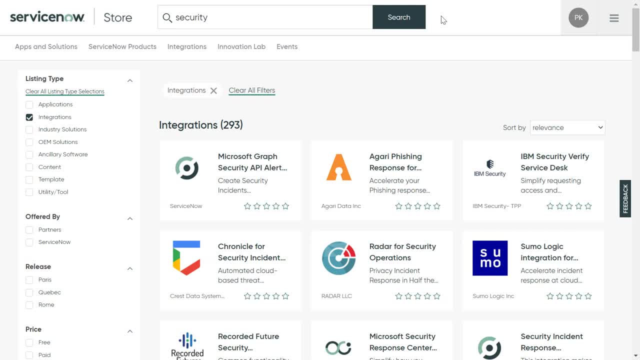 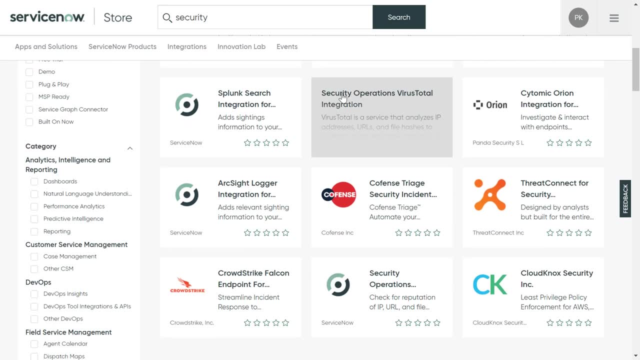 There are out-of-box integrations with security sensors and SIEM platforms such as QRadar, ArcSight, LogRhythm, Splunk and Splunk Enterprise Security. Threat intelligence programs are also very helpful for security incident handling, saving analysts times with automated threat lookups. 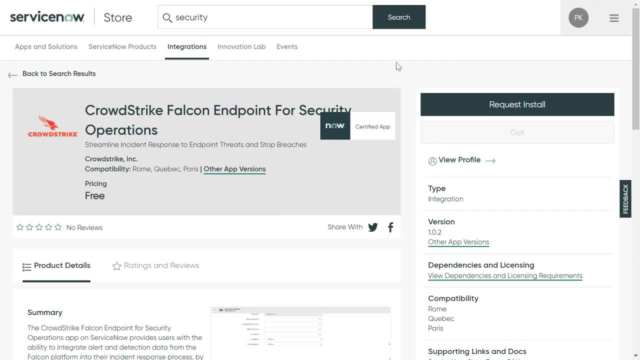 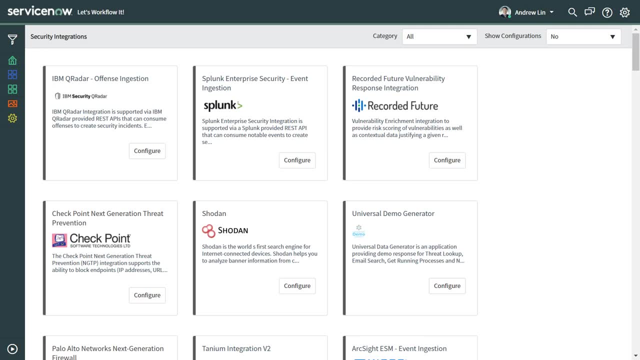 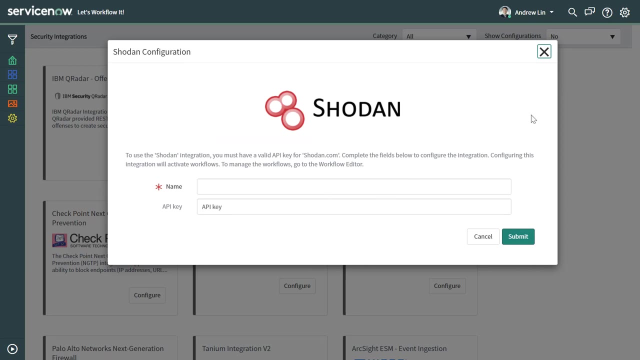 Customers can request their integrations from instances right here in the store. Once installed, these applications can be configured inside your ServiceNow instance. Some simply require API keys, such as Shodan here, while others have more options like setting a schedule or adding filters to the data we want. 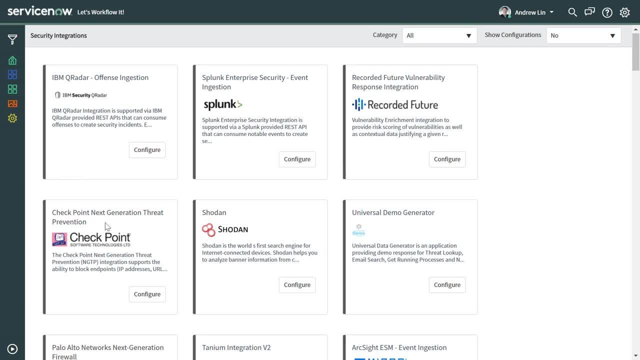 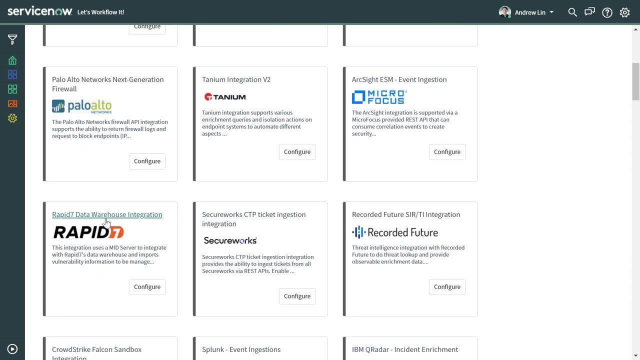 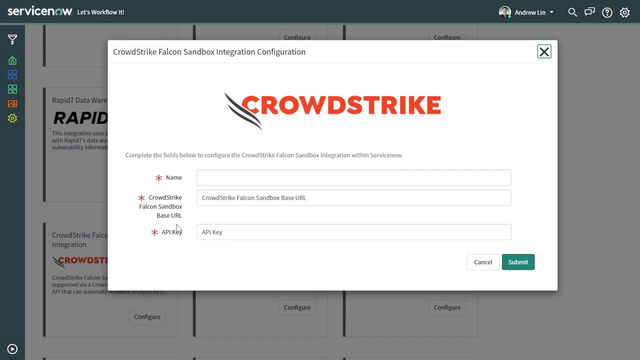 Phishing emails come in a variety of different forms, and often they include malicious attachments. Analysts can now submit malicious attachments for in-depth malware analysis using the CrowdStrike Falcon Sandbox integration. The integration allows for both manual and automated submissions, as well as a variety 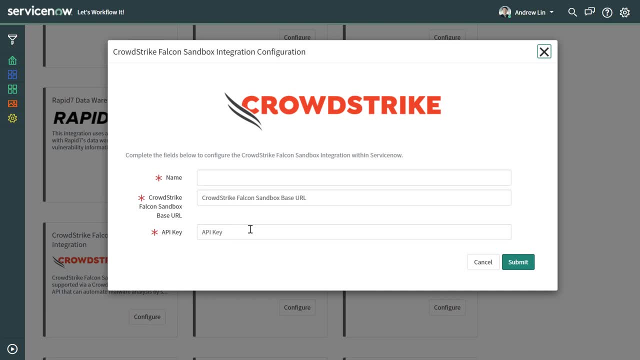 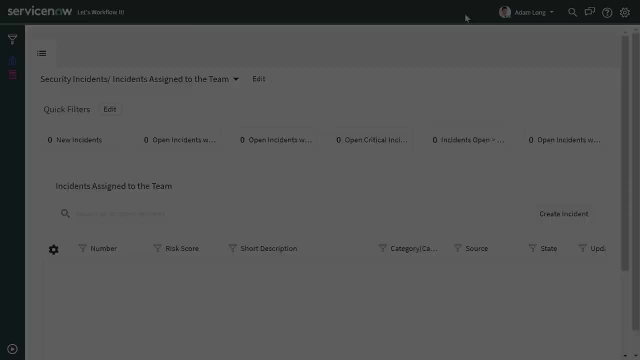 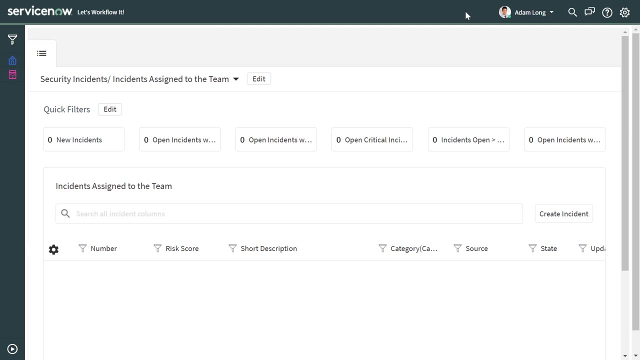 of other settings. This provides the possibility for Sandbox submission results to be completed during the triage process and ready when the analyst first opens the security incident. Let's see how the platform helps incident handlers like Adam Long here get work done faster and more effectively every day. 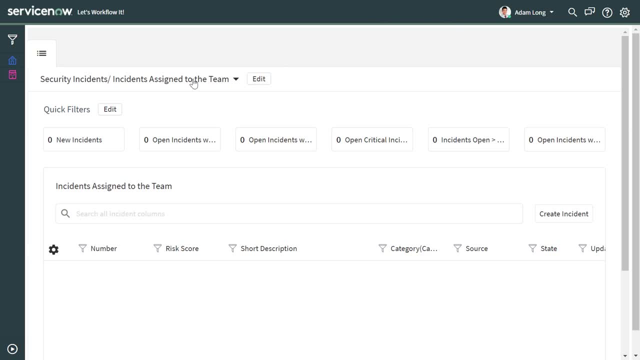 From here, Adam sees incidents that are assigned to him or his team. With customizable filters, he's able to quickly navigate the pool and review automated triage details. It looks like this. It's a great way to get started. It looks like there's a new incident here today. 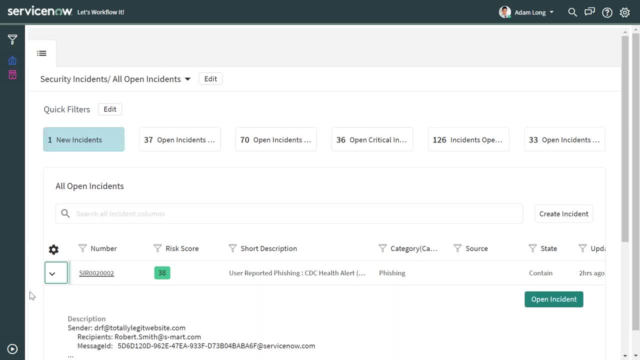 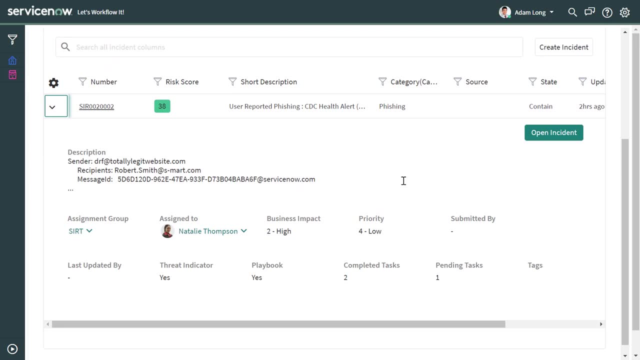 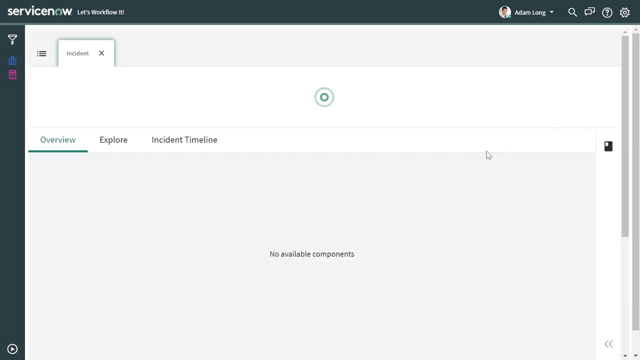 Adam can take a closer look with Peak View. This one has a high business impact, a confirmed threat indicator and a machine learning analysis saying suspicious. Clearly this one's important, so Adam opens it in a new tab. Adam can keep multiple incidents opens at a time. 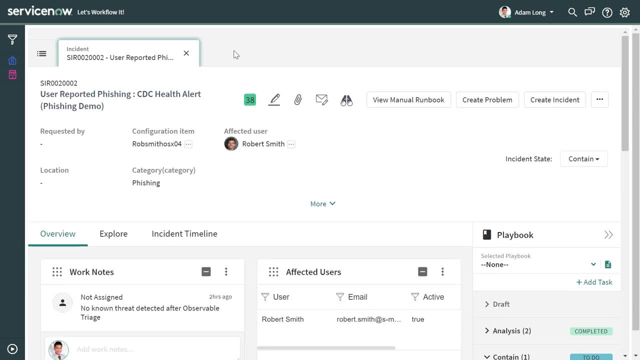 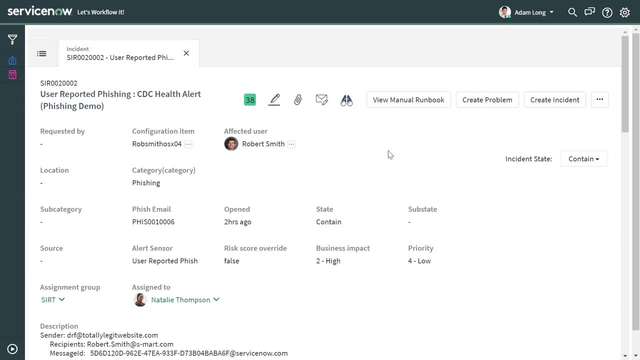 if he needs to multitask while automations run. It looks like this is a phishing report from Robert Smith. In the old days, Adam used to have to watch an inbox and do all this manual triage, threat analysis and calculate risk manually. 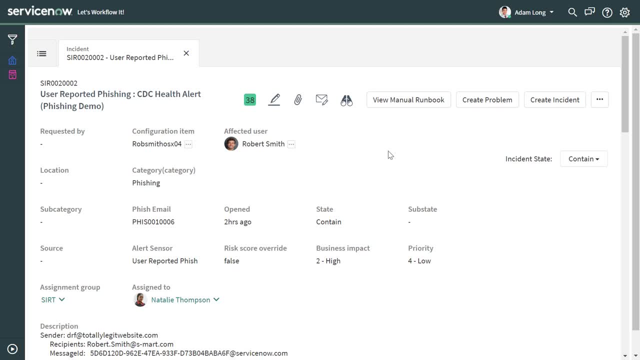 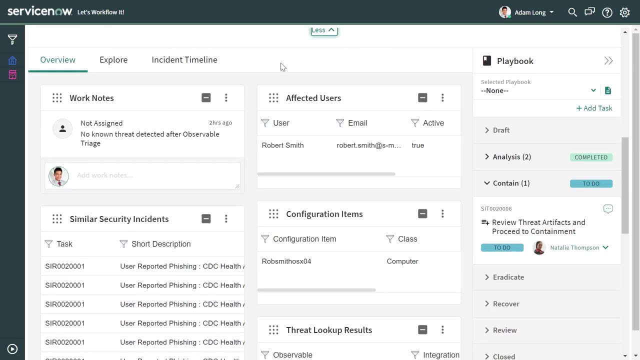 But now when he logs in, all of that has been done for him automatically. Employees can simply hit a Report Phish button in their mail client or forward a suspicious email, and ServiceNow will do all of that work automatically. In the Overview tab, Adam has his favorite widgets arranged. 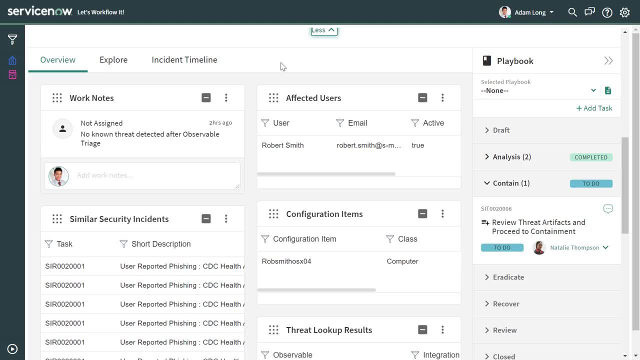 so he can have a quick look at all relevant info for the incident. Every analyst can personalize this tab and move them around as they see fit. One of Adam's favorite tools is this Similar Security Incidents widget, which shows all security incidents that have technical similarities to this one. 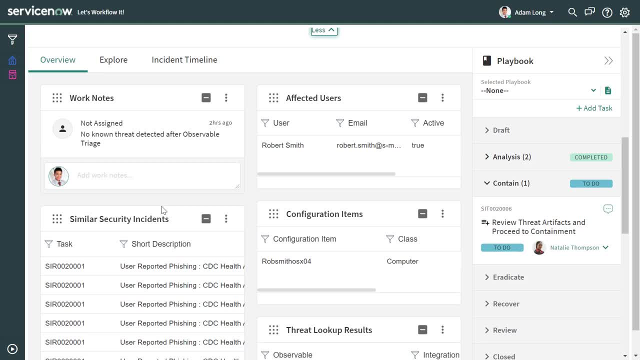 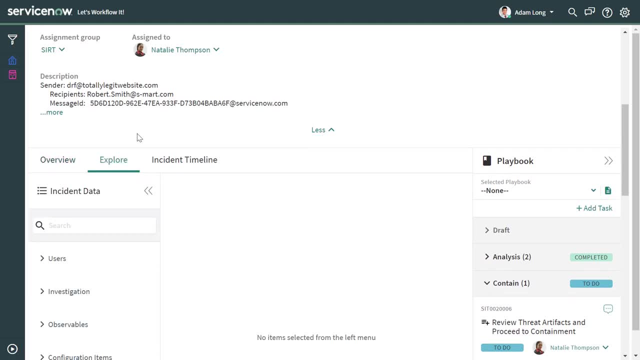 such as the same URL, IP file name, file hash or email subject. With the Explore tab, Adam can dig into any of the details, such as the URL, IP, file name, file hash or email subject. With the Explore tab, Adam can dig into any of the details. 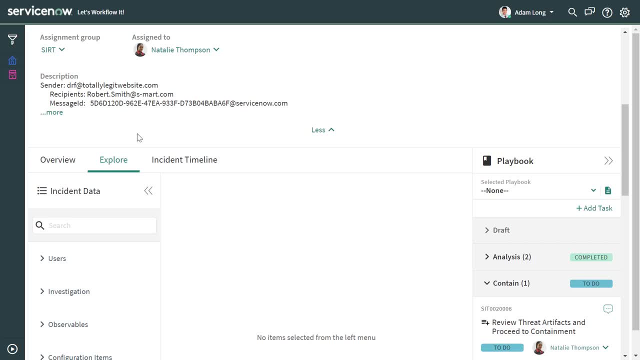 such as the URL, IP, file name, file hash or email subject. with the Explore tab, Adam can dig into any of the details and this security incident, such as who is affected by it. In this case, it is Robert Smith. 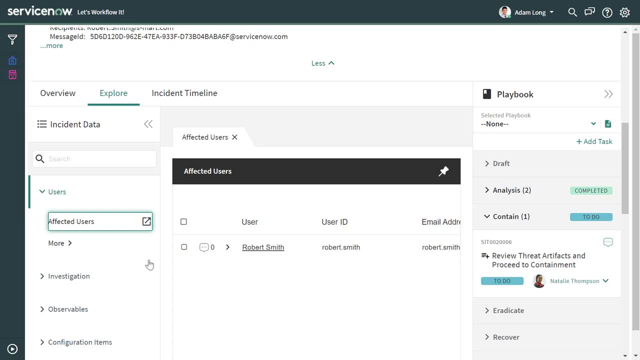 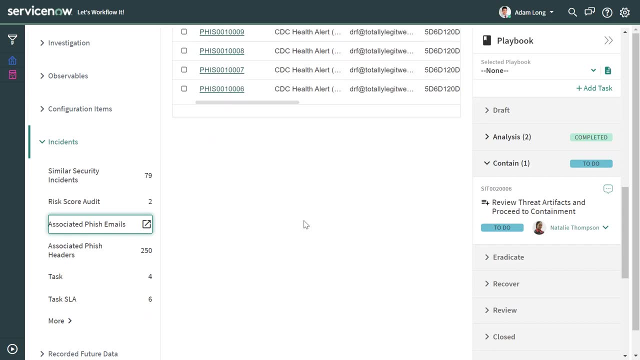 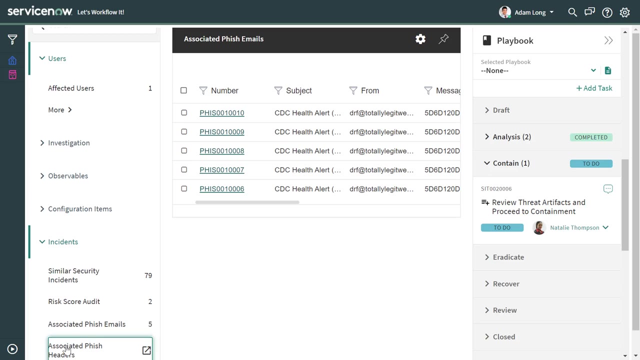 the first person to report this phishing email. Adam also benefits from deduplication In this case. this email has been reported by a number of individuals seen here. Optionally, deduplicated reports can create child incidents instead. All of the email headers are parsed out. 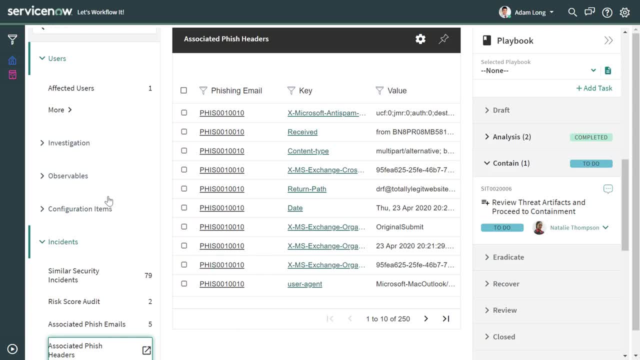 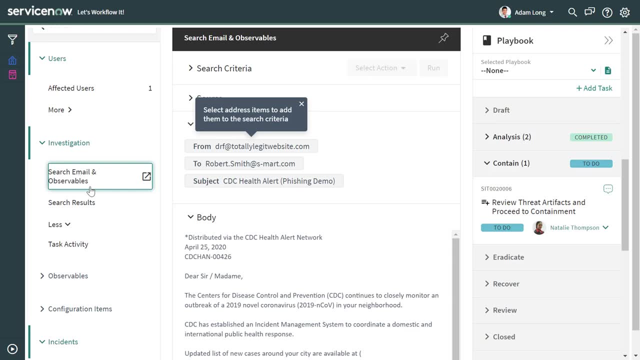 as structured data and shared data as well, and these can be used in automation. Next, Adam takes a look at the email that was reported and sees a familiar pattern. These COVID-themed phishing emails have been coming in a lot lately. Parsed observables end up here: 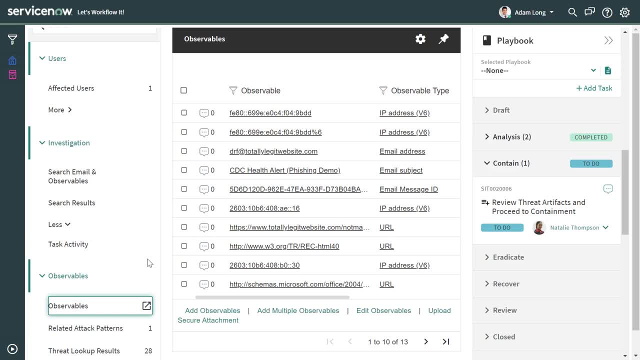 along with whether or not they're deemed malicious from threat lookups that have already run upon the creation of that incident. Running these manually is also pretty trivial as well, and Adam doesn't need to be an expert in dozens of products to leverage all of his organization's threat sources. 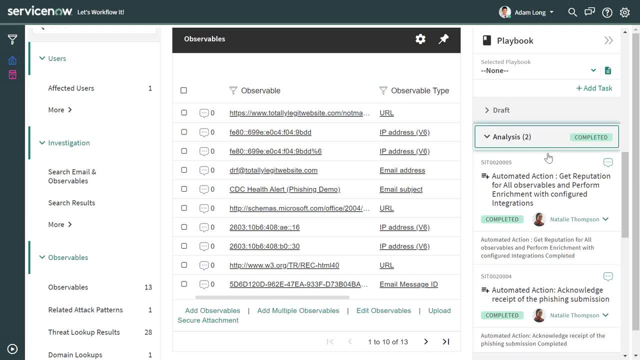 Here on the right we see the playbook pane. Adam can see where he is in his team's security or automation playbook posture for a phishing response. Security incident response comes with dozens of flows like this one, and they're configurable via the graphical editor and flow designer. 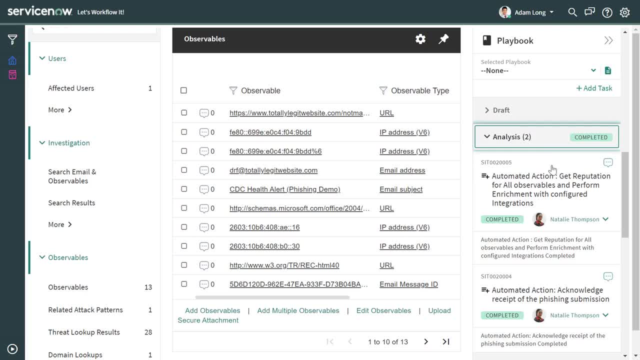 When tasks are created, they end up on the right over here We can see where automated lookups were executed and completed Again, steps and any detailed guidance here are completely configurable, making it easier than ever to architect and use security playbooks. 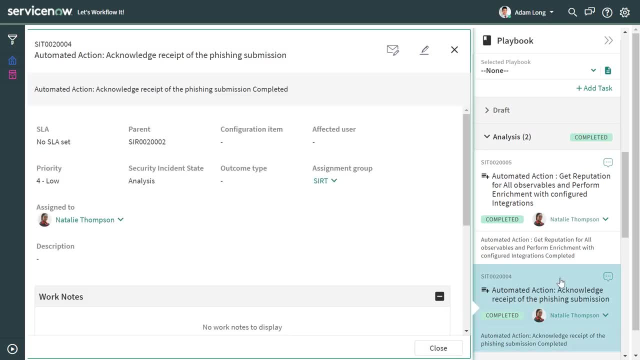 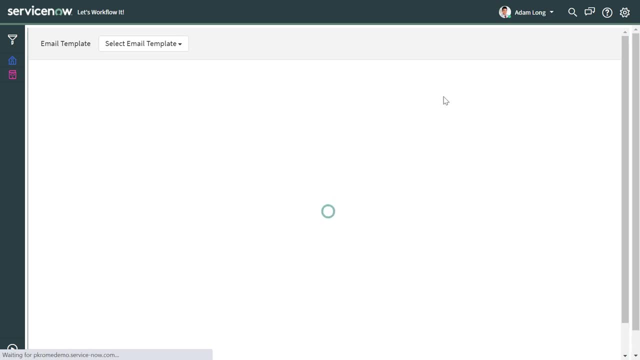 For example, the threat intelligence orchestration we discussed has taken place and the person who reported the phishing incident was automatically contacted via email to thank them for their submission. Sometimes this kind of work is less predictable, so, of course, any of the things. 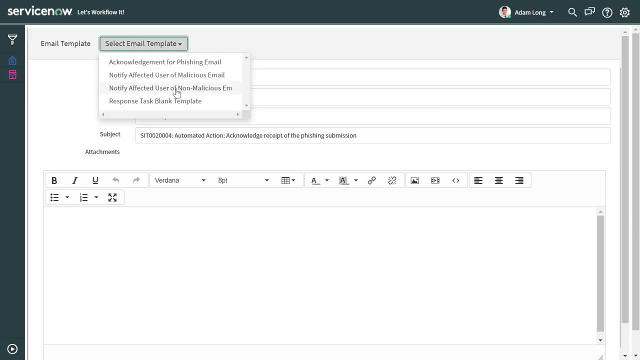 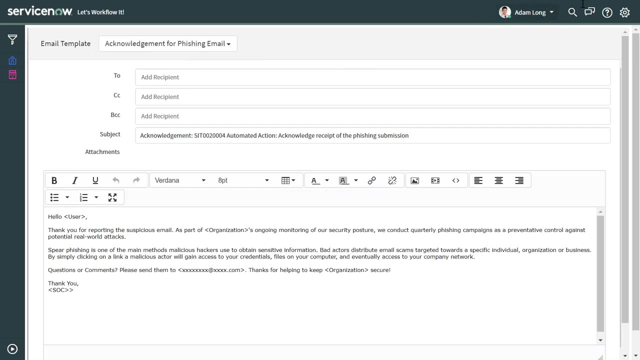 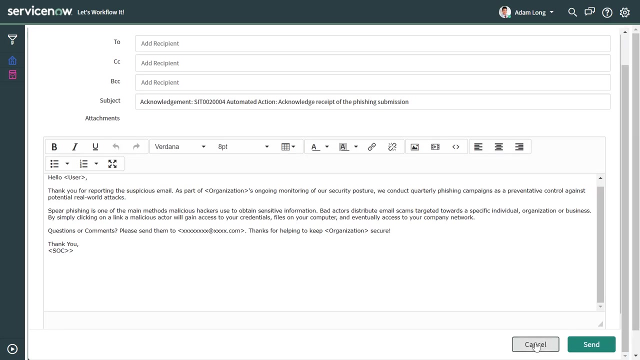 that are automated steps we show can also be done manually in the UI. In the case of sending an email, templates like these can help facilitate this kind of communication. ServiceNow can send mobile app notifications, text messages and also integrates with messaging platforms such as Slack and Microsoft Teams. 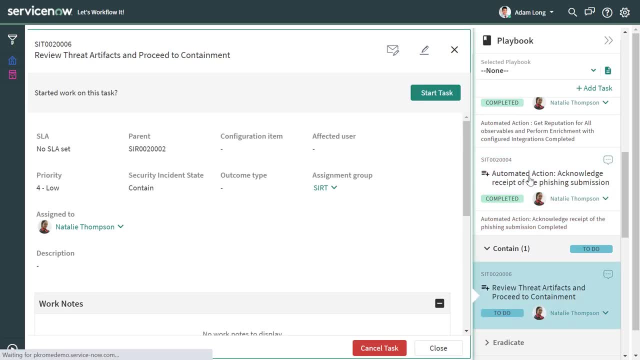 Now that these first automated steps have completed, Adam only needs to review and confirm the findings. Once he does, the playbook will take care of the rest: finding and deleting these malicious emails across all users' inboxes. performing firewall blocks for phishing URLs. 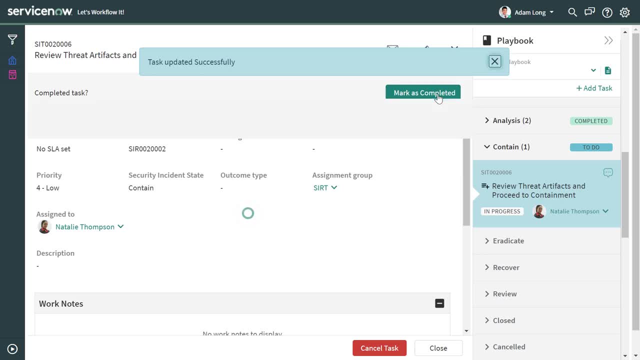 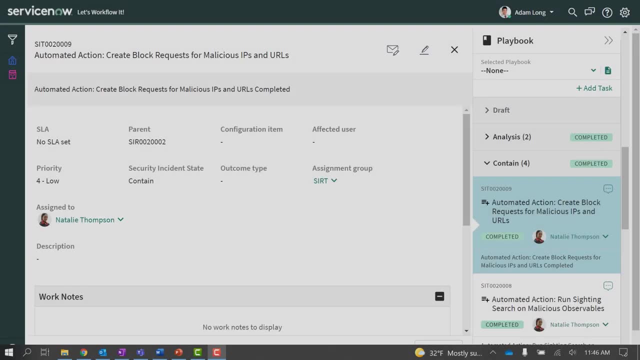 and searching SIEM and log platforms for any other potential victims. These following actions are documented inside the child task. here Adam agrees with the automated analysis, so he completes this task to fire off the second half of the playbook. While these steps are being automated in the background, 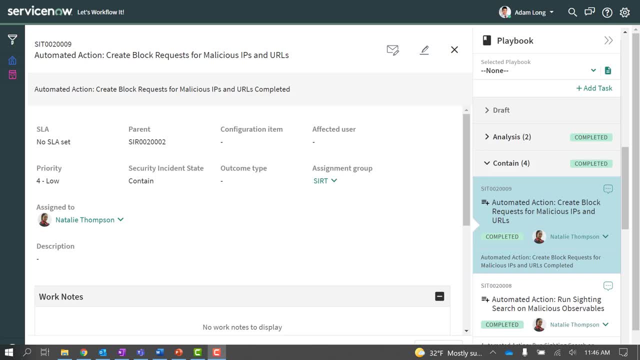 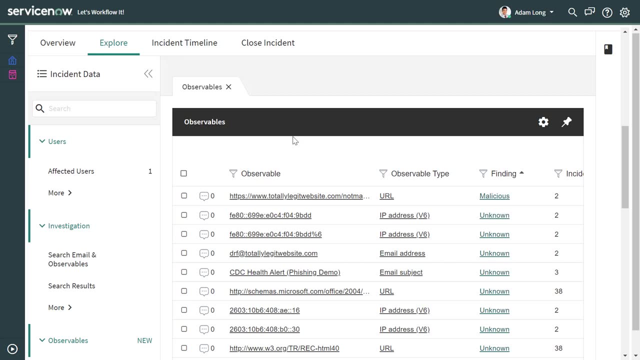 let's quickly review the first half of the playbook. Let's quickly peek at how they are done manually. To perform a firewall block request, we pick an IP or a URL and check the box next to it, Select block request and then run it. 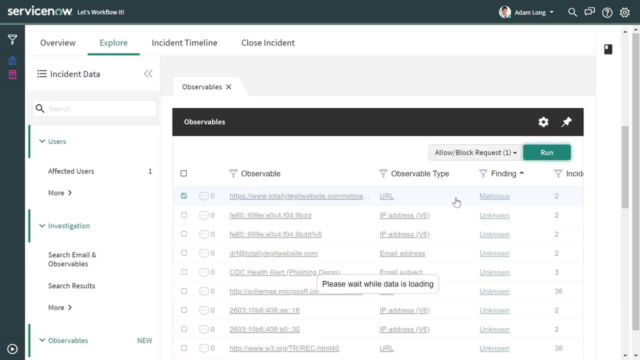 And then we can choose which vendor or list to request the block with. This works the same way with citing search to find any matching logs and can search for matching emails and delete them. like this, Select the best app to define the desired host of the network. 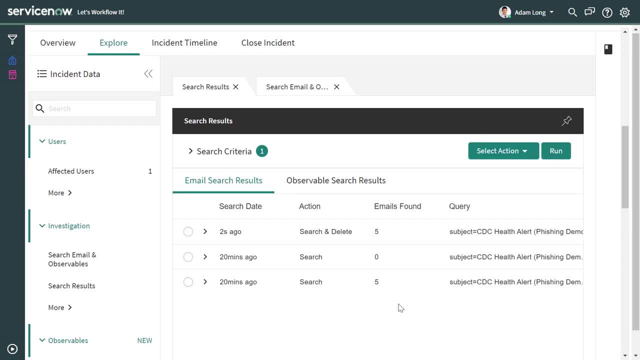 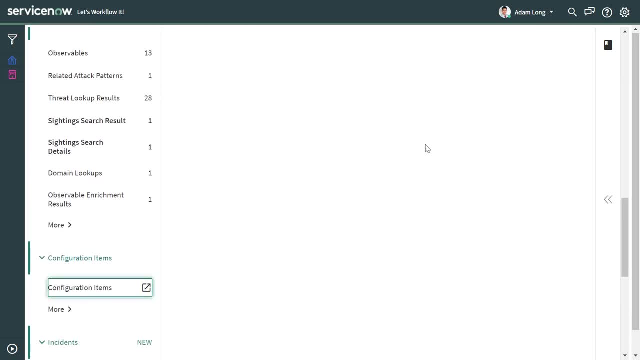 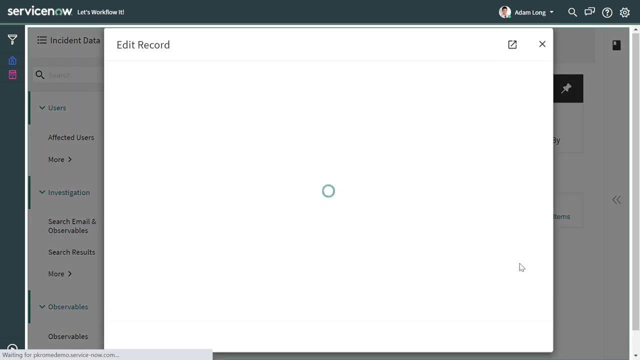 and enter the address of the address. Then the results can be viewed here. If you have an asset in play, there are even more automation options. For example, Adam can add one to the incident and isolate the host from the network, if needed Here by clicking on edit configuration items.